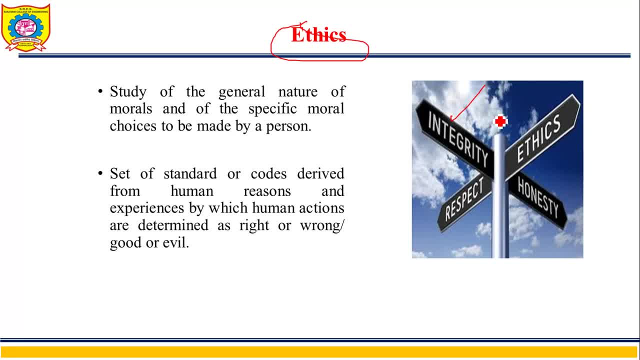 So in this you can see that different words are given here. The first word is Integrity, the second word is Ethics, then Honesty and Respect. So all these constitute for Ethical Decisions. okay, So it is a study of general nature of morals and of the specific moral choices made by the person. 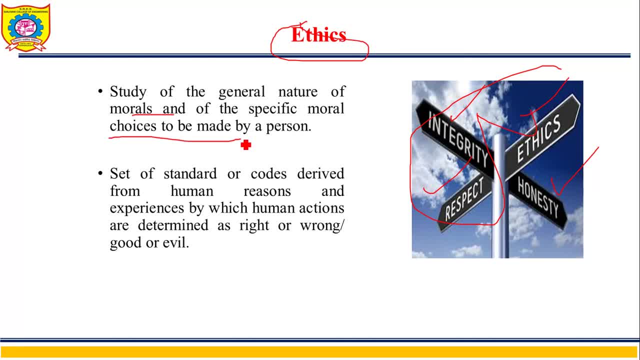 Now, what are the choices? The choices are: what is good, what is bad, what is good, what is bad. So this is the study of all these things, And it is a set of standards or codes derived from the human reasons. 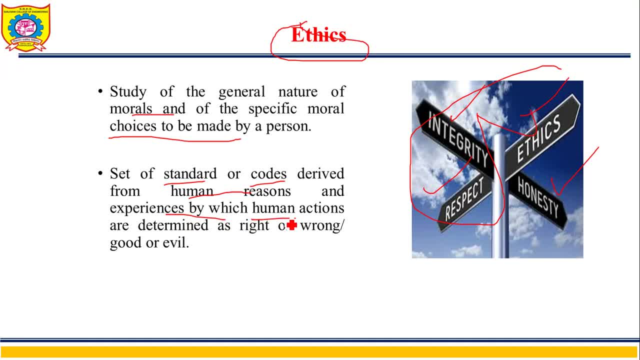 Where experiences, which are experiences by human actions, Are determined as right or wrong. So what it has in it? it has the meaning of Ethos. Ethos is a Greek word And from there Ethics word derived, And our 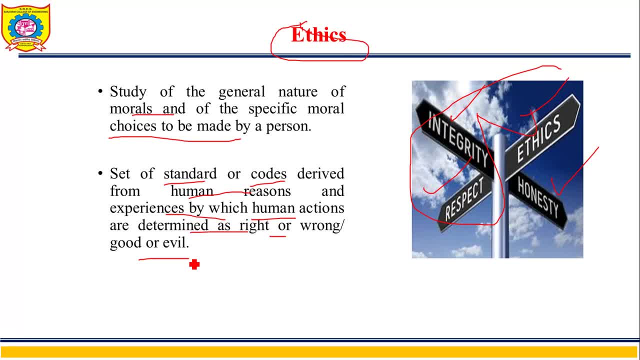 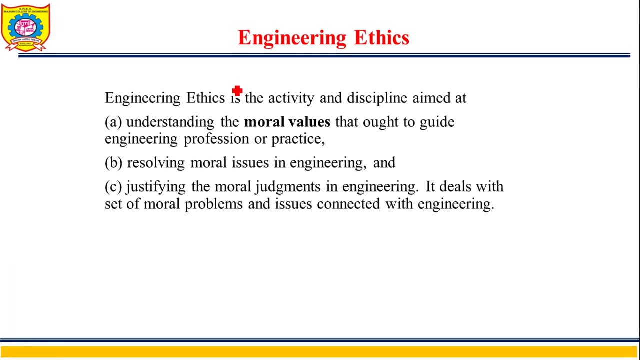 About our Acharya and Vicharya, about good or bad, What is right, what is wrong. It gives us knowledge about this. This, This is what this word teaches us. now, if you are coming to the next point, the next point is engineering ethics. if you look at this, 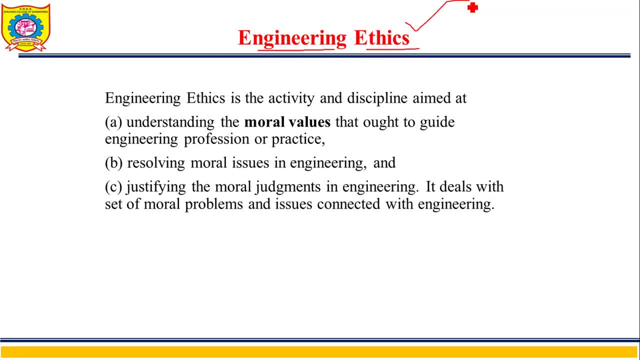 particular word, key ethics to me, but the chalga key it is kaki. it is some sort of you know what is good, what is bad, what is right, what is wrong. it's all about all these things and this ethics we have to also follow in the engineering. when, uh, engineers get the job, they have to follow this. 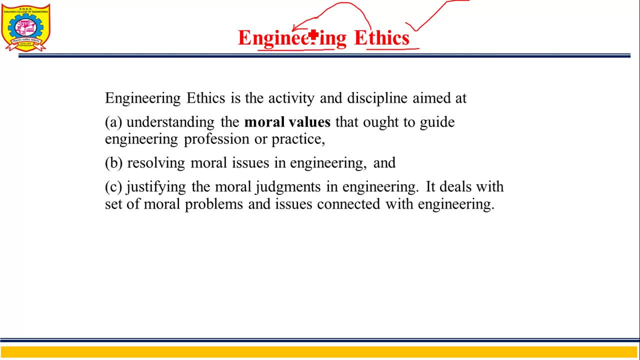 type of ethics in the uh in their profession also. so engineering ethics is the activity and discipline aimed at understanding the moral values. so even though, if you are working in a very, very good organization or multinational company in the engineering profession, whatever moral issues come there, we have to resolve them and 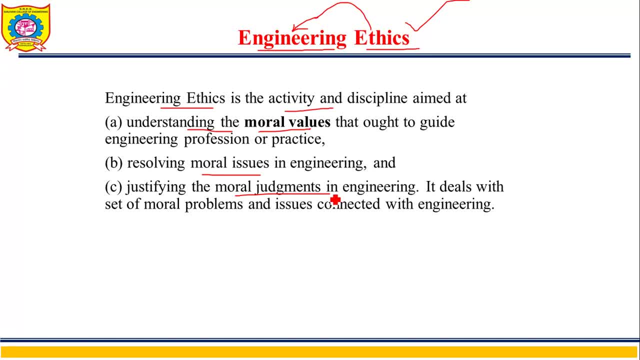 we have to justify moral judgments in engineering ethics. okay, so it's all about solving the problems, moral problems and issues connected with the engineering. so we have to keep in mind that in engineering ethics we have to understand moral values and we have to utilize it in engineering. 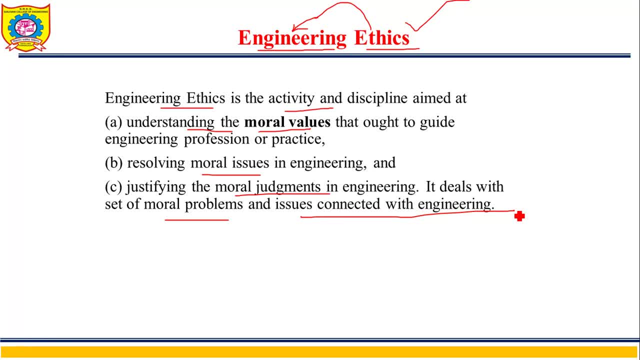 we have to resolve them and any moral judgment that, aligned with the knowledge, we have to justify it. and with this źertification, Jonas Justice judgment, we have to solve the moral problems and issues related to the engineering and because of it, it has to be solved. this is engineering ethics. 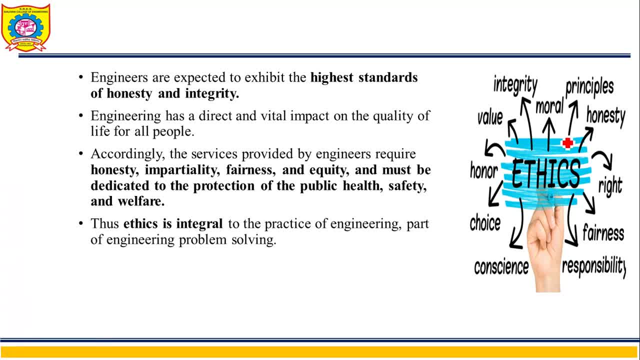 now, if you, if you are looking to this particular ppt, you will see Ethics. now you have understood the meaning of Ethics. ok, Here there are different words like Integrity, Morals, Moral word, Principle. There is word Honesty, There is one word Right, There is one word Fairness. 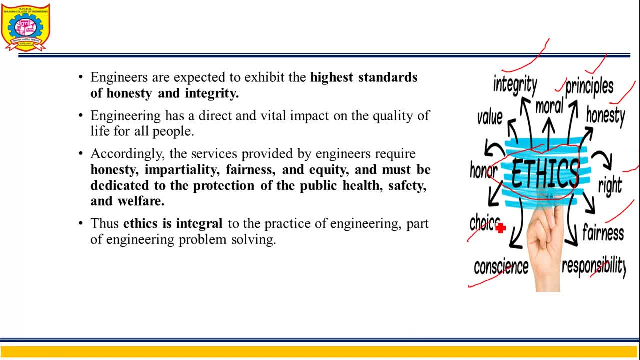 Responsibility, Conscious Choice, Honor, Value. Value means Price or Value. Integrity means Accuracy, But here, in case of Human Values, we have to consider that Integrity is related with Honesty, Truth, and Honesty Morals means Niti Principles. Here We can say that this is also very important. 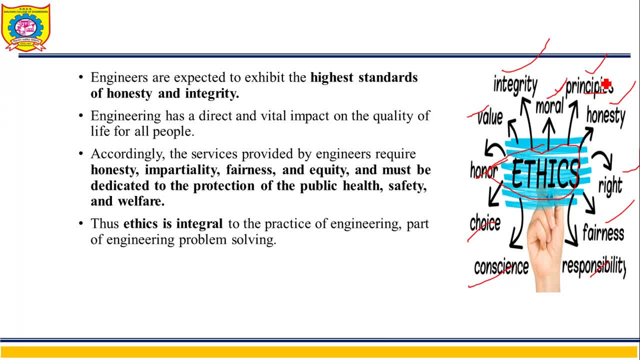 And in case of Engineers, There is, you know, we have to follow the principles and guidelines Into the profession also. Honesty. Honesty is also a very important thing when you are designing any product or when you are in any professional organization. Right What is Right? 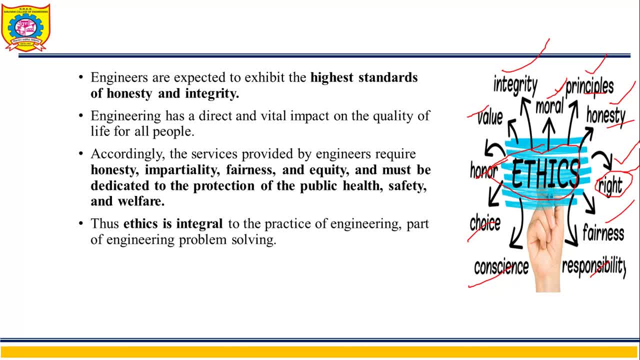 You know. so right means Adhikar, It is my right. Ok, After that, there is Fairness, which we can say, that Nishpakshata, which we can say: Responsibility is here. Responsibility, Consciousness, means Satvik. Wisdom, which we can say: Choice means we have an option. 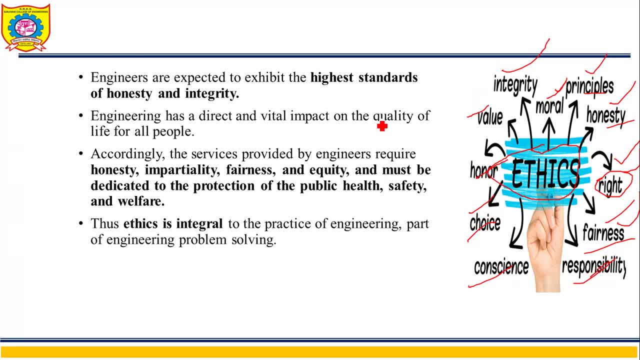 Honor, Values and Integrity. So Engineers are expected to exhibit the highest standards and Honesty and Integrity, Higher standards of Honesty and Integrity. So whenever you are going into any particular professional organization or a multinational company, So there we have to give the highest standards of Honesty and Integrity. 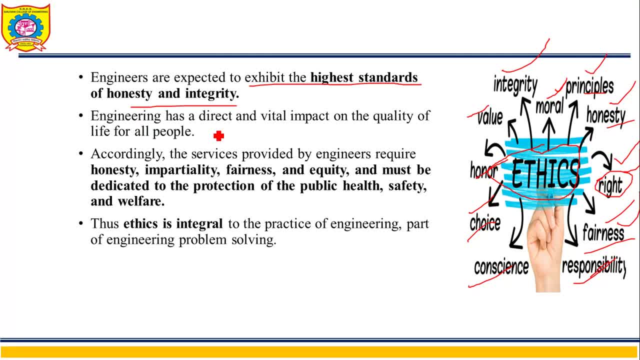 Ok, And Engineering has a direct and vital impact on the quality of the life of people. Like you can see that Everywhere there are different types of products around us. Around us, Here you can see mobile laptop, television, washing machines, refrigerator. We all are surrounded with the engineering technologies, engineering equipment. 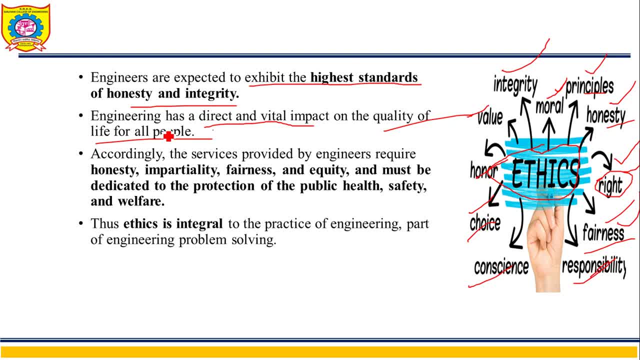 So all these things have a very big impact on our life. Accordingly, the services provided by the engineer requires Whatever engineering profession comes in the services And there comes honesty, impartiality, fairness, equity, And we have to think about public health, safety and public welfare. 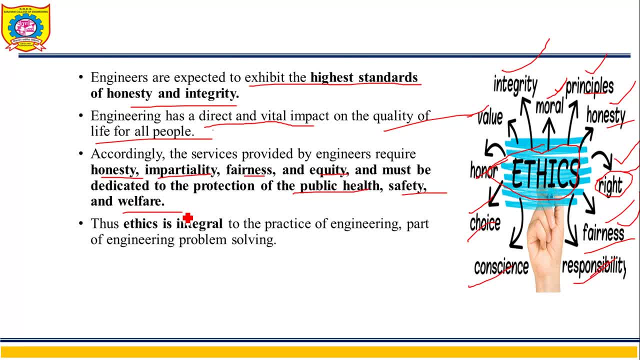 So all these things we have to implement as an engineer When we are designing the product or when we are launching a product into the market. Thus, ethics is integral. That is why all these services that are provided, So we integrate all these and follow the ethics. This is the practice of engineering. 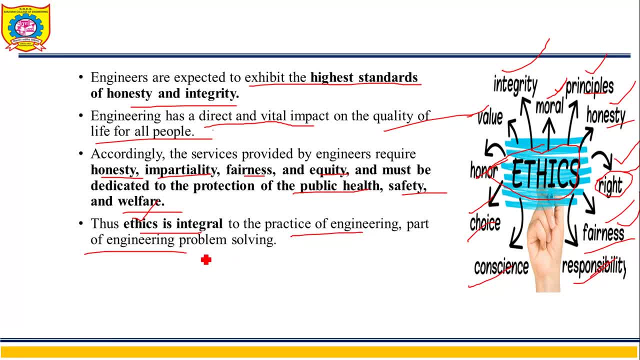 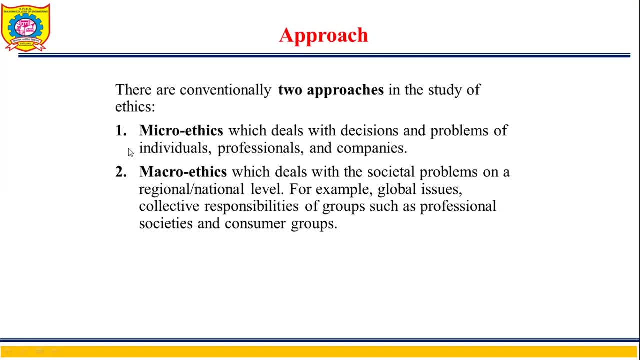 And in this way we can solve the engineering problems in the professional life. So if you look at this approach, Actually, if you look at this particular thing- There are basically two types of engineering approaches. The first approach is microethics- Now, micro means very, very small In this particular- and the second part is macroethics.